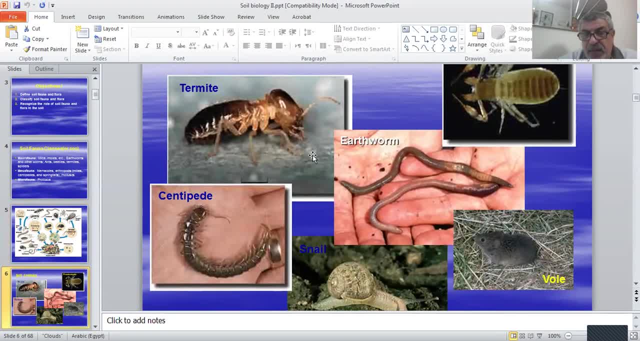 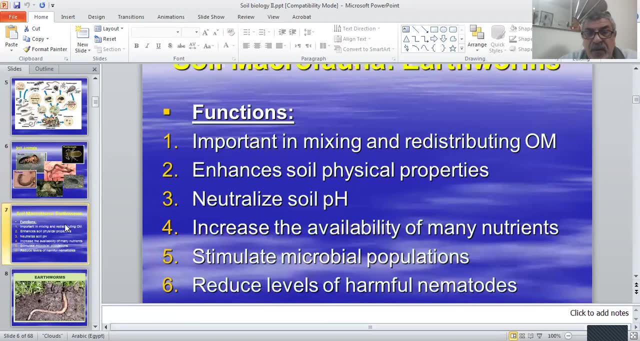 This also the pictures of some of the fauna in the soil, The functions of, the functions of of fauna or earthworms in the soil that we have so many functions. Number one, important in mixing and redistributing organic matter, inheres the soil physical properties. 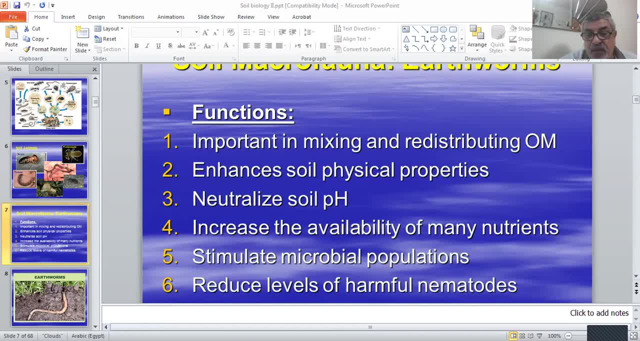 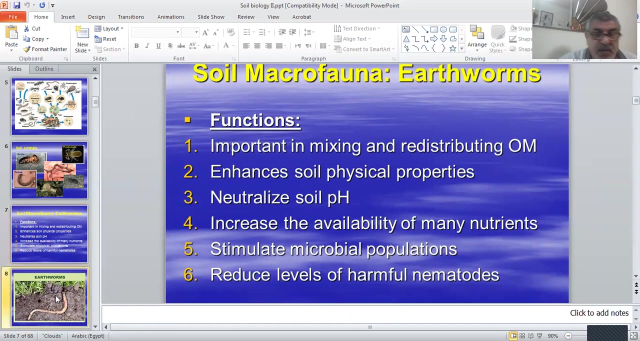 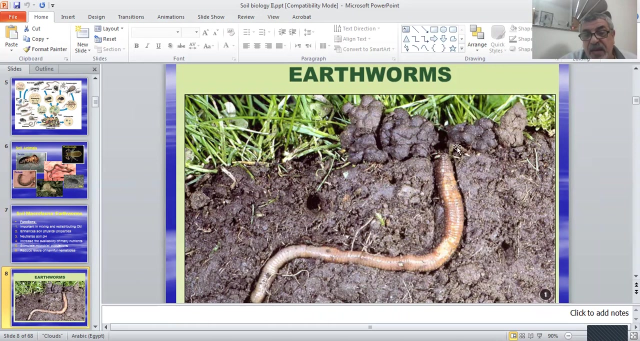 neutralizes soil pH, increase the availability of many neutrons, stimulates microbial population, reduses a level of harmful nematodes. So it is a very important function for the earthworms in the soil. Yes, this is the picture of earthworms in the soil and it borrows the soil and makes tunnels like this. 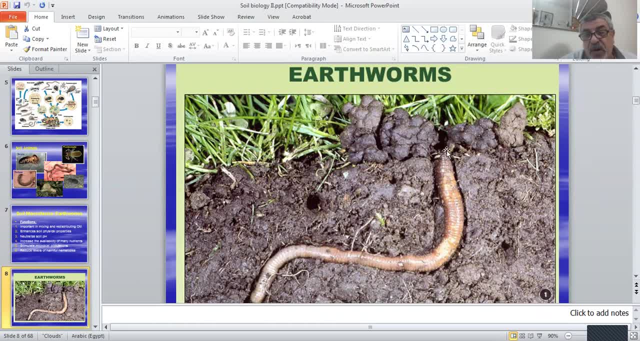 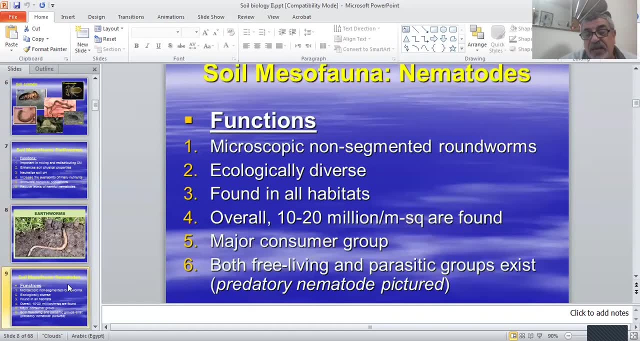 And this is very important for many things, as we mentioned. Besides, it aerates the soil and encourages the exchange of soil air. About the nematodes, or soil mesophonic nematodes, it's a function that is microscopic, non-segmented around the world, ecologically diverse, found in all habitats. 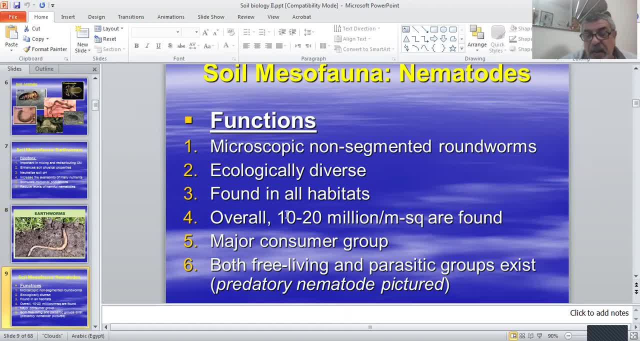 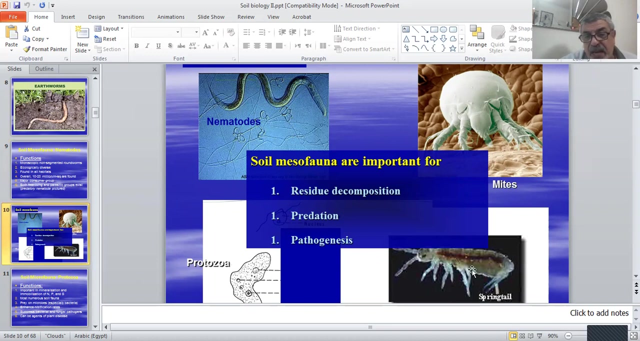 Overall about 20 million- It's counted about 20 million per square meter- A major consumer group, both free living and the parasitic group, Some of them beneficial and some of them parasitic. These are the mesophonic types: the nematodes, the protozoa and the mites. 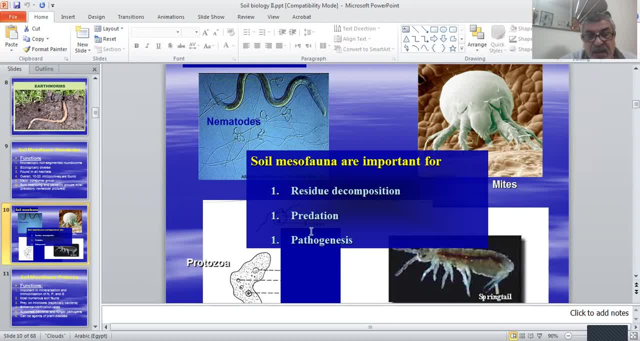 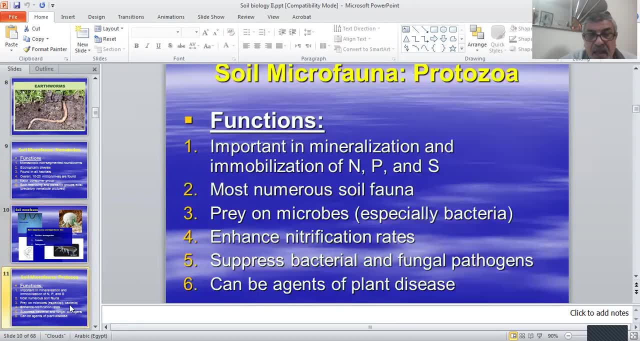 The main functions are here: important for residual decomposition, validation and pathogenesis For the protozoa. it is important in mineralization and in polarization because it is the main source of nitrogen, phosphorus and sulfur. Most numerous soil fauna prey on microbes, especially bacteria. 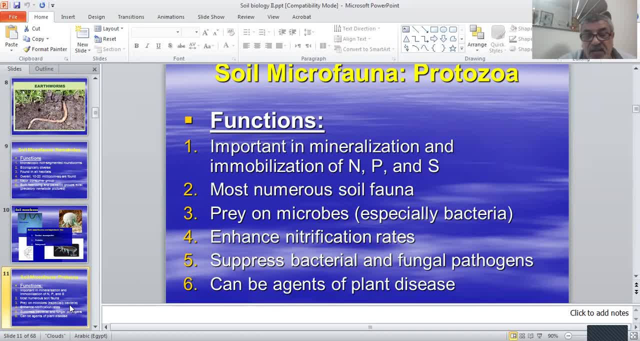 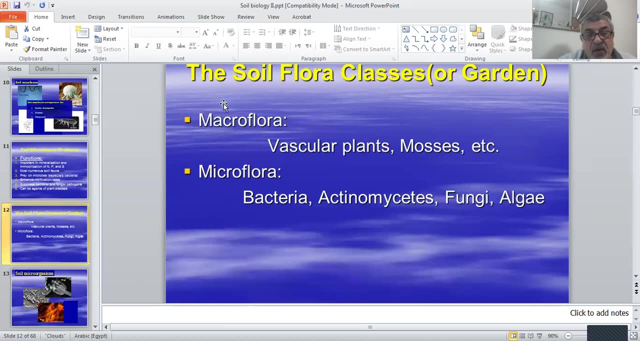 and hence its nitrification rates, suppresses bacterial and fungal pathogens. It can be an agent of plant disease. The soil flora classes- we have macroflora and microflora. The macroflora is the normal plants. The microflora contains bacteria, actinomyces, fungi and algae. 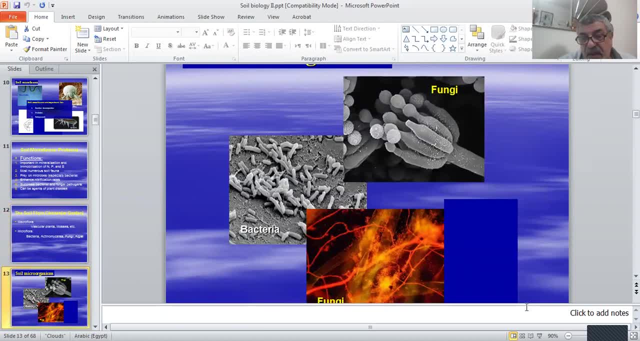 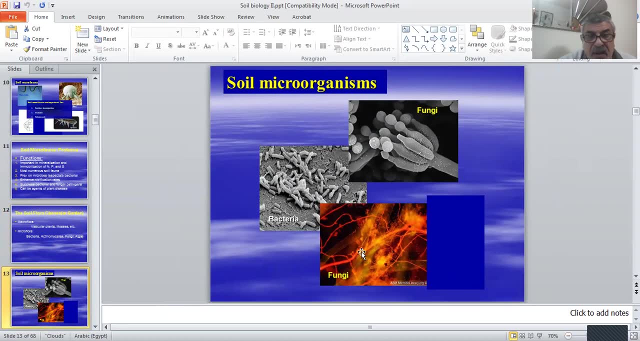 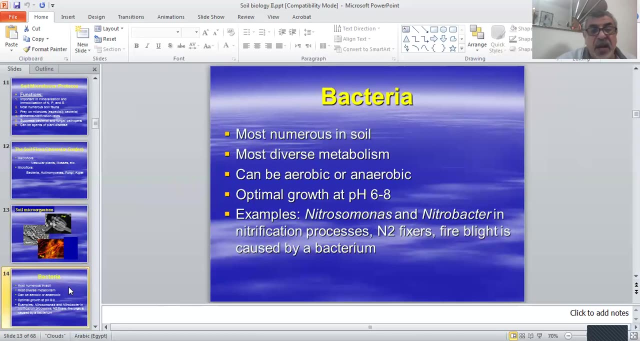 These are the photos of microflora and microorganisms in the soil: fungi, bacteria and algae. About bacteria: they are the most numerous in the soil, Most diverse metabolism can be aerobic or anaerobic. Optimal growth at pH between 6 and 8.. 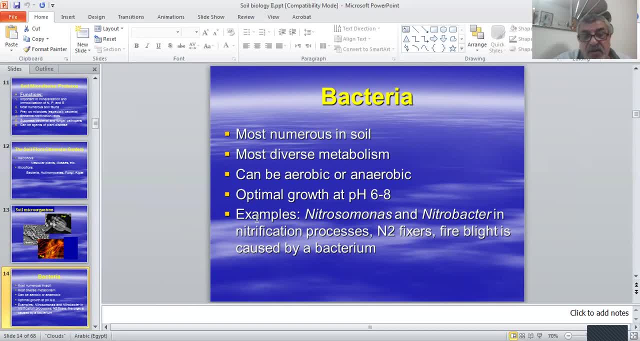 This is very important. Examples of bacteria is Nitrosomonas nitrobacter, which is, which are very important in nitrification process, And also nitrogen fixer, and and Bacterium azotobacter. Soil is alive. 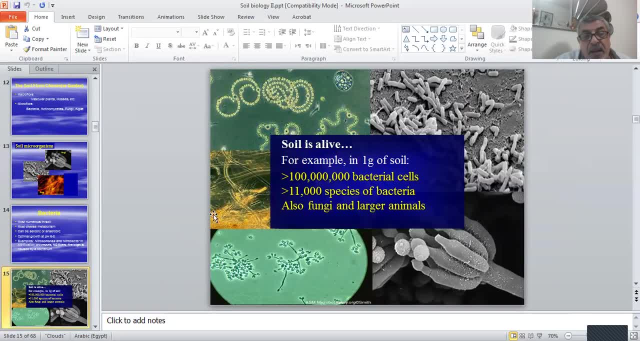 We must know that soil is alive, not dead. One gram of soil contains 100 million bacterial cells, 11,000 pieces of bacteria, also fungi and larger animals. So soil is alive and we must keep it alive. About actinomyces: 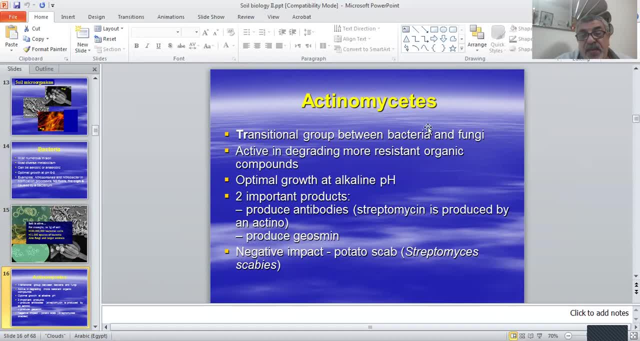 It is a transitional group between bacteria and fungi Active, integrating more resistant organic compounds. Optimal growth at alkaline site. Take care of this. Actinomyces have optimal growth at alkaline pH. It produces important product like antibodies And 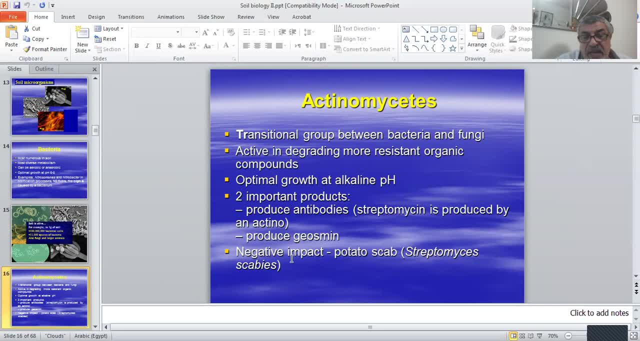 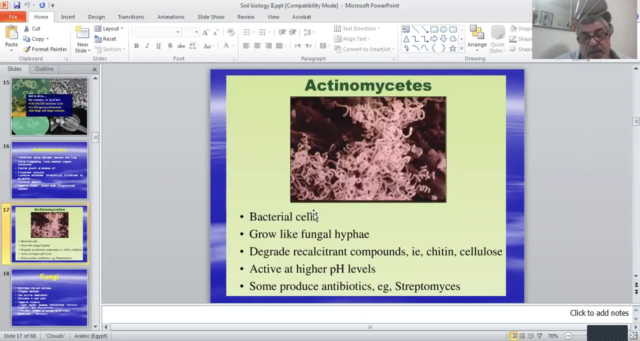 Ziojusmin Negative impact on potato, as streptomyces, scabies And the brown disease- This is the actinomyces. It is a kind of a bacterial filamentous bacterial cell- Grow like fungi. fungi Degrade the 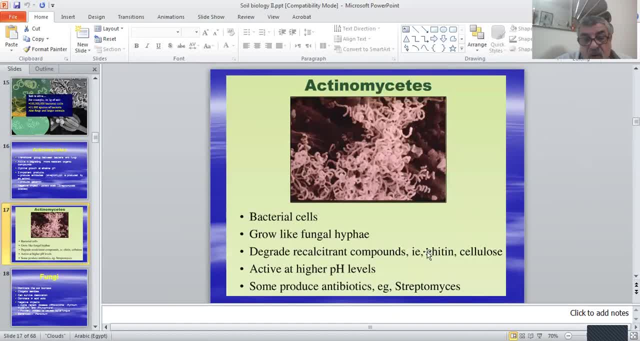 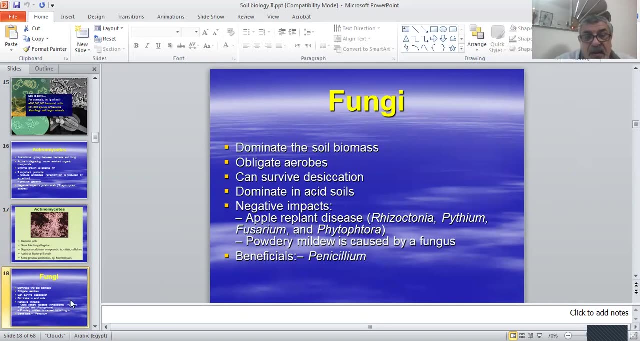 decarcerant compounds- chitin, cellulose and active at higher pH levels, and some produce antibiotics and streptomyces For the fungi. it dominates in soil biomass. Obligate aerobics can survive desiccation, dominating acid soil. Fungi prefer acid soil, acid condensation, low pH. 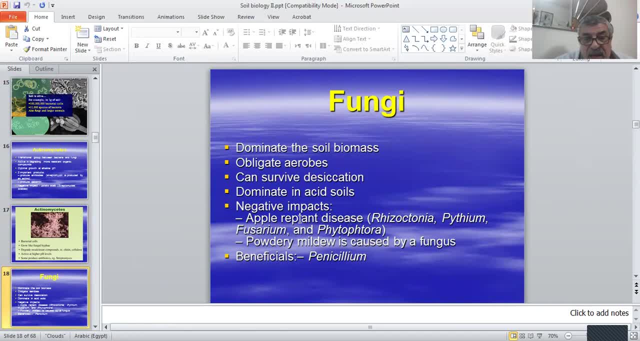 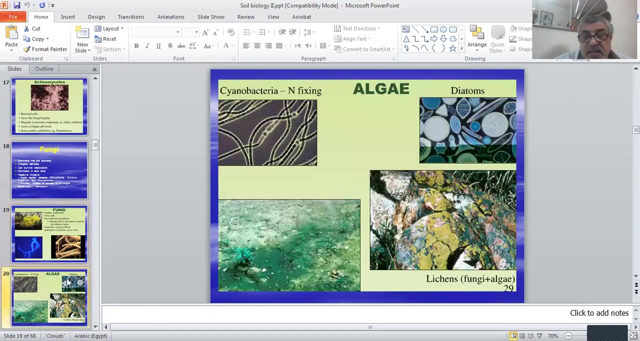 Negative impacts make diseases to apple and some fungal diseases for other plants Beneficial. some of them are beneficial, like penicillium. Penicillium is very important in producing antibiotics. This is a photo of some fungi and this is photos of some algae. 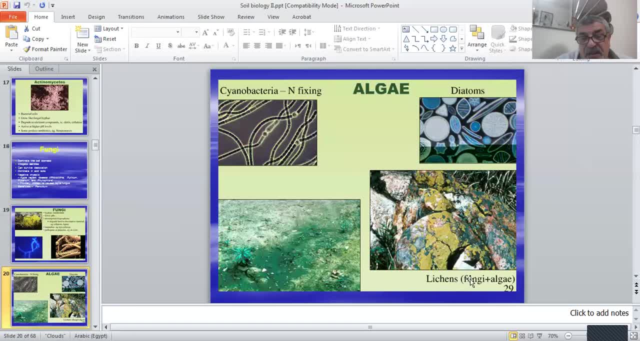 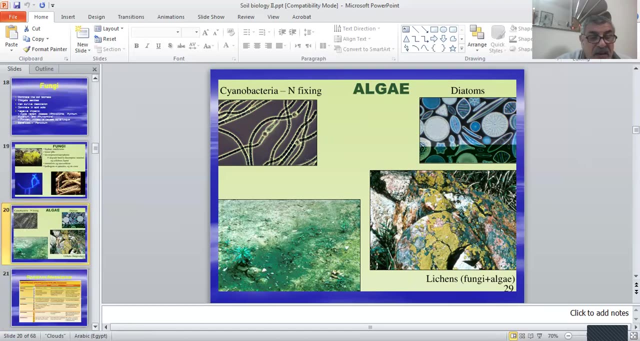 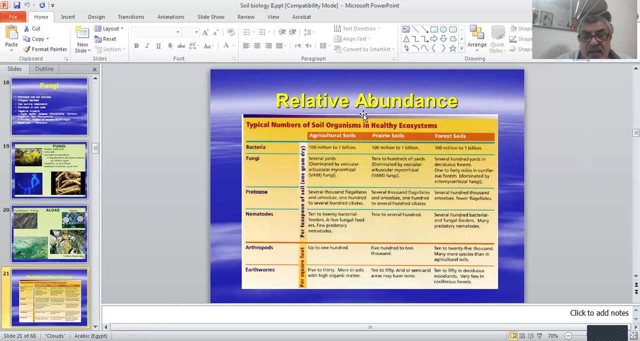 cyanobacteria, the atoms, All of them can make photosynthesis and form sugars, which is motivating the other creatures to be activated. The relative abundance of all the groups we mentioned according to the number bacteria is found in: the highest number Fungi, protozoa, nematodes. 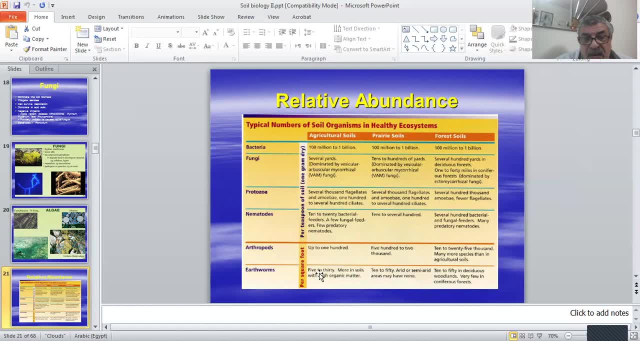 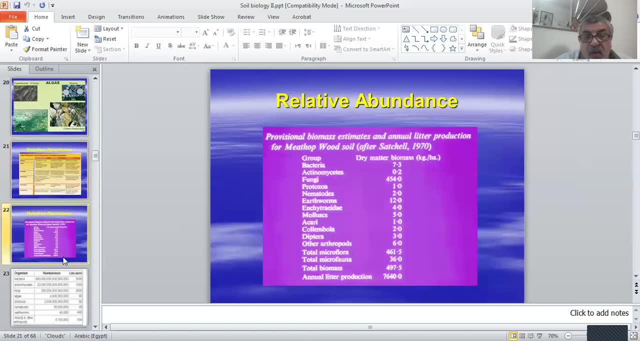 anthropodes, esteroids, and these are in descending order According to the numbers, as we notice here, according to the weight, the relative abundance. according to weight, the most dominant one is fungi, As you see here, fungi, followed by